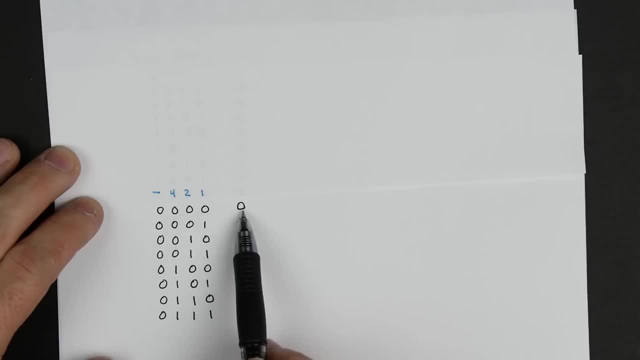 Of course, if we have all 0s, 0,, 0,, 0, 0,, that's equal to 0. And then if we have a 1 in the 1's place, that's equal to 1.. 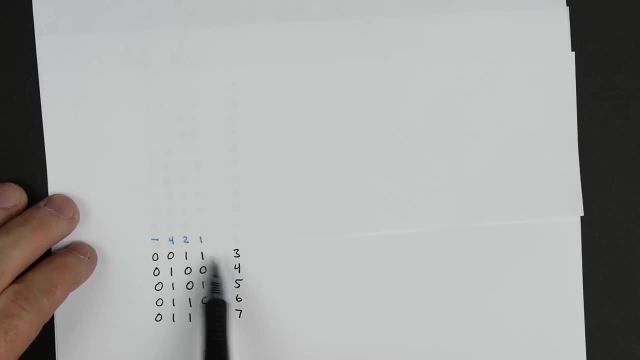 We have a 1 in the 2's place, that's equal to 2.. A 2 and a 1,, that's equal to 3.. And then, of course, a 4 is 4.. A 4 and a 1 is 5.. 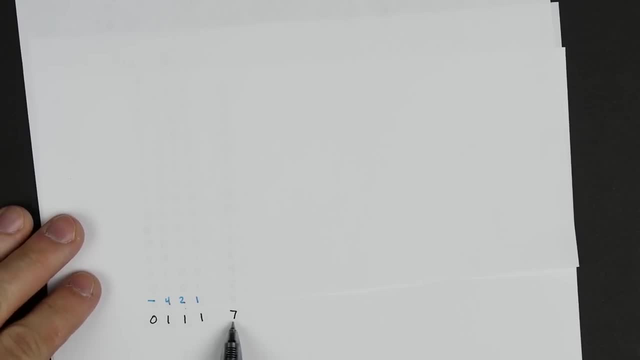 A 4 and a 2 is 6.. A 4, a 2, plus a 1 is 7.. So that's simple enough. And then if this first bit here is indicating our negative sign, then we can go backwards too. 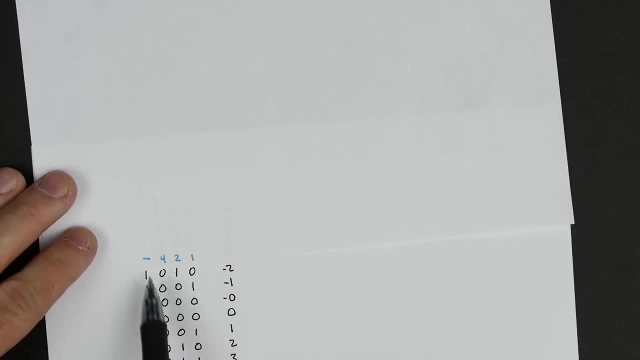 So if we have a negative 1, that's negative, 1. A negative, 2.. A negative 2 and a 1 is 3.. And then a negative, negative, 3., Negative, 4. A 4 and a 1 is 5.. 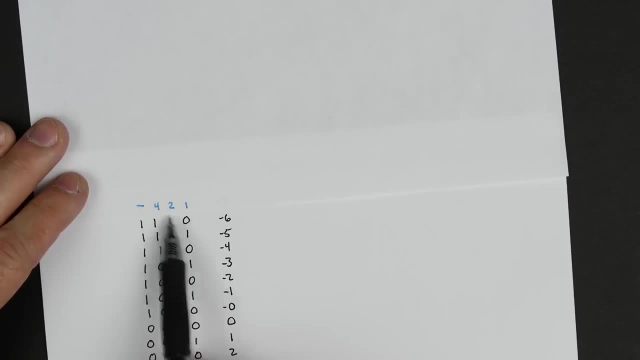 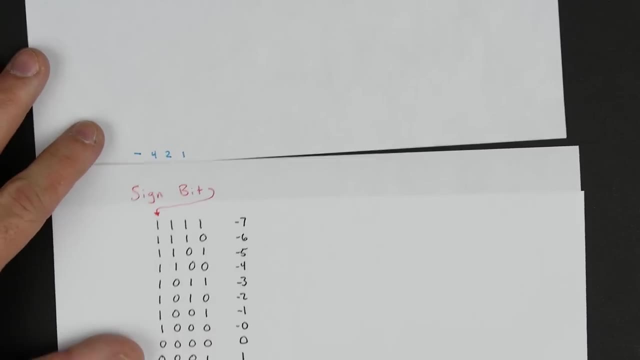 With a negative is negative 5. A 4 and a 2 is 6.. So this is negative 6.. And then a 4 plus 2 plus 1 is 7. And that's a negative 7.. And so this is our sign bit. 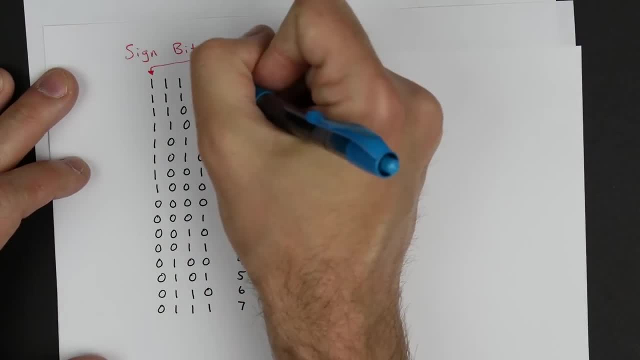 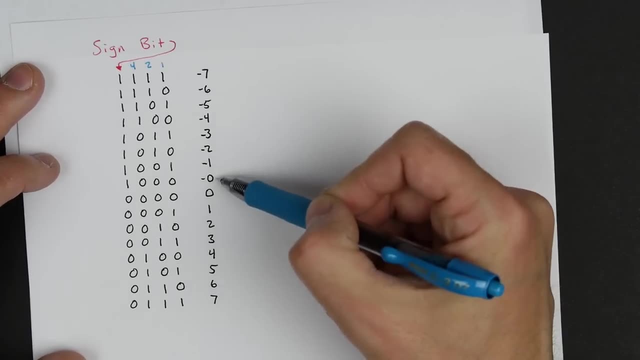 And so this first bit is our sign bit, and then these other bits are just our 1,, 2, and 4 place. Simple enough. A couple weird things about this, though. One is that you'll notice there's a negative 0, right. 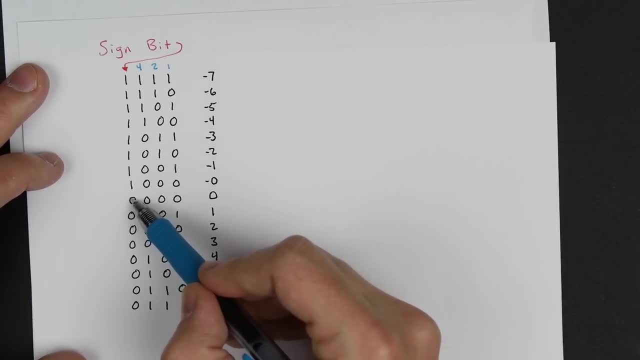 Because you can have 0,, 0,, 0, and then it can either be a 0 in the sign bit place or a 1 in the sign bit place. So you can have you know there's a difference between 0 and negative 0. 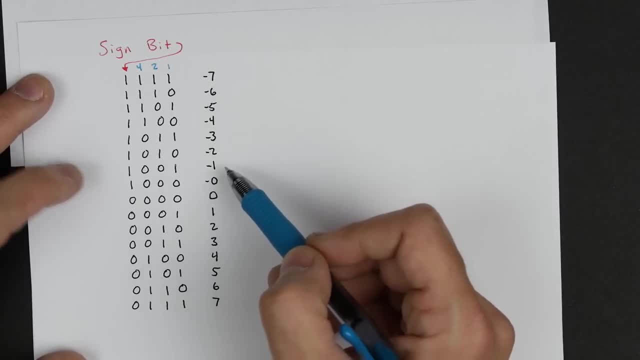 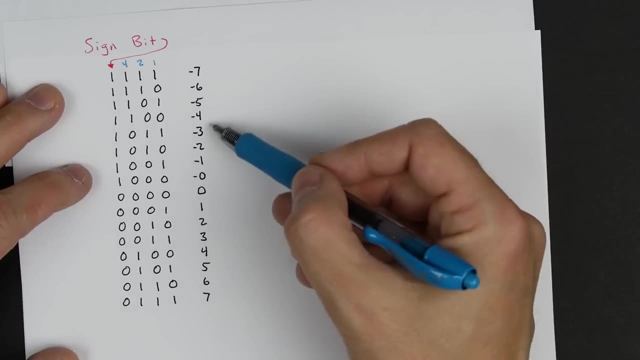 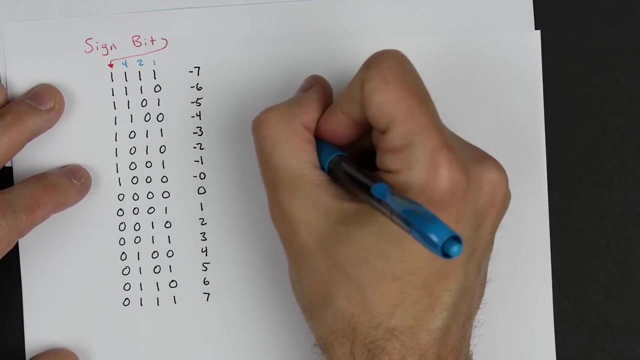 So that's kind of weird. The other thing that is maybe a little bit inconvenient- and we'll look at some other approaches that don't have this problem is if you try to add these things together, things get kind of weird. So let's say we want to add a 5 and a negative 5.. 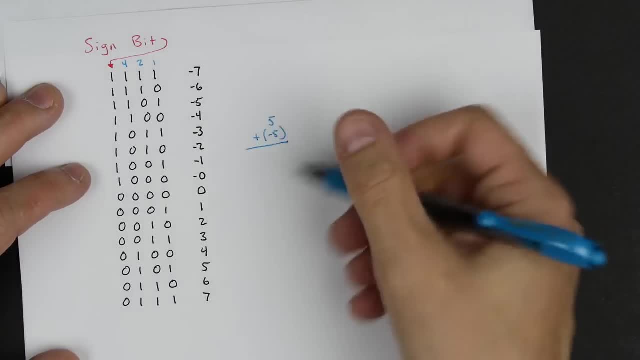 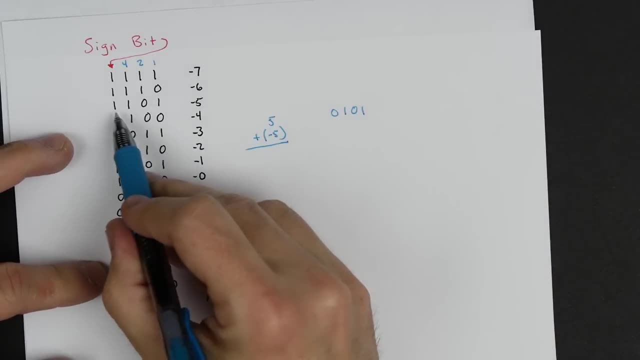 So normally 5 plus negative 5, you would expect to get 0.. Simple enough, But here, if we look at 5, 0, 1, 0, 1.. And negative 5 is 1, 1, 0, 1.. 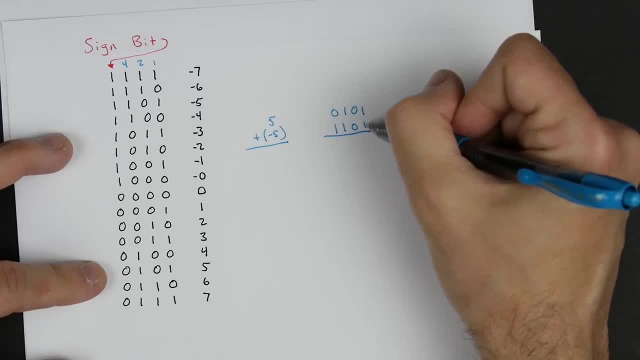 If we add these together, 1 plus 1 is 2, which would be a 0, and then carry the 1.. 1 plus 0 plus 0 is 1.. 1 plus 1 again is 2, but we'll put that as a 0 and carry the 1.. 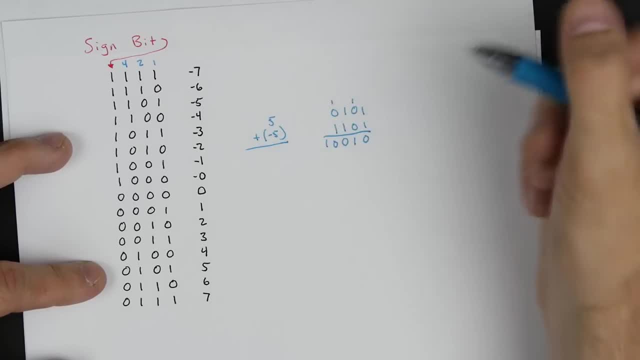 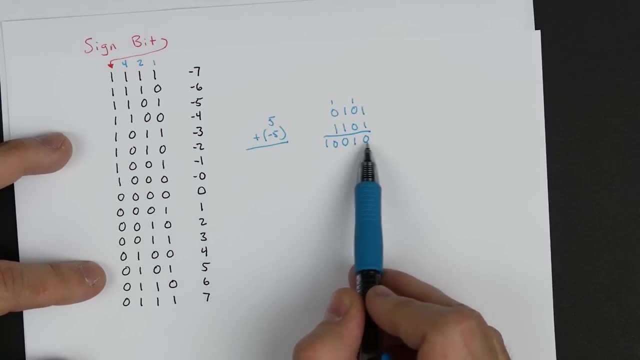 And then here, 1 plus 1 again is 2, so 0 and carry the 1.. So in this case, what we're seeing is 5 plus a negative. 5 is not 0. It's 0, 0, 1, 0, which, well, and we have a carry. 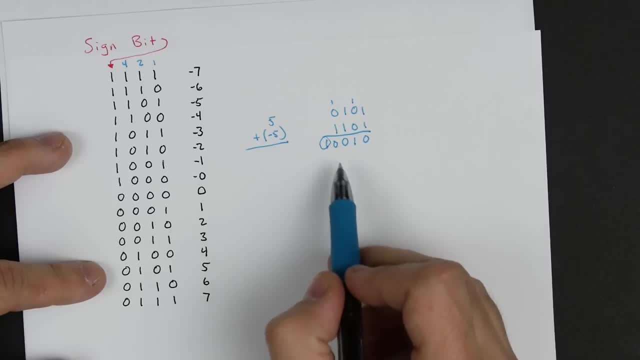 So we have a carry coming out of this 1 bit that we don't. you know, if we're working with 4 bits, we're going to ignore this carried bit, And so we have 0, 0,, 1, 0,, which is 2.. 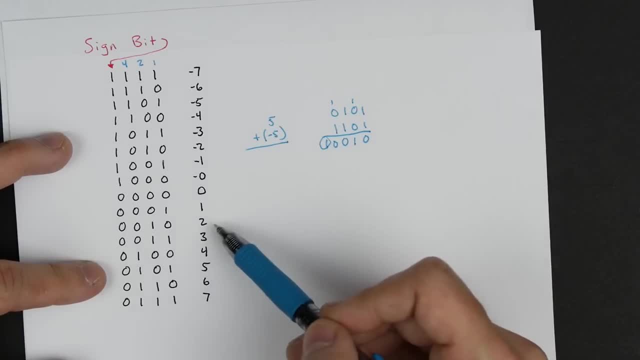 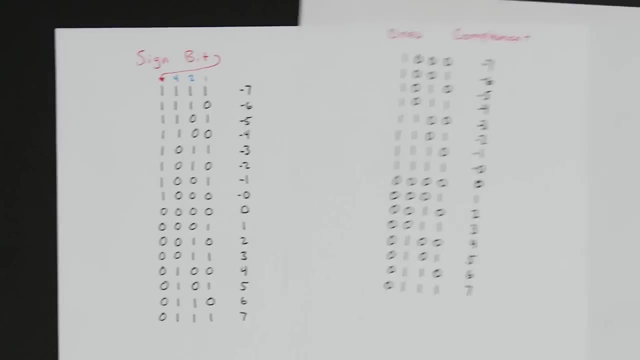 So that's kind of weird. If we're adding 5 and negative 5, we wouldn't expect to get 2.. And you can try adding some other things here. It doesn't work. So let's take a look at another scenario here. 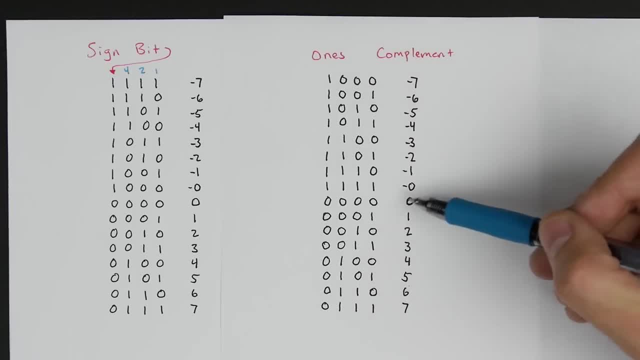 This is called one's complement. What this is is, again: everything from 0 to 7 is the same same as we saw before, And this first bit here is all 0s, so we know that these are all positive. 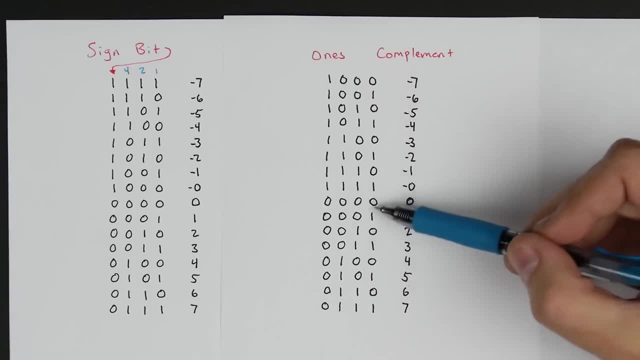 But what we do for the negative numbers is we actually just flip all of the bits. We take the complement of all of the bits. So you know, 2 here is 0, 1, 0. Well, 0, 0, 1, 0. 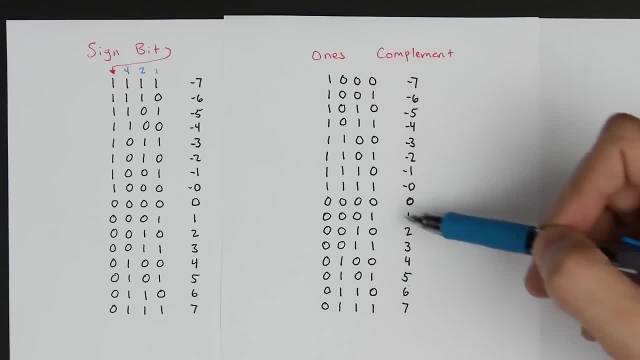 Negative 2 is 1, 1,, 0,, 1.. So we're just flipping each of those bits. So we flip the 0 for a 1.. We flip the 1 for a 0.. We flip the 0 for a 1.. 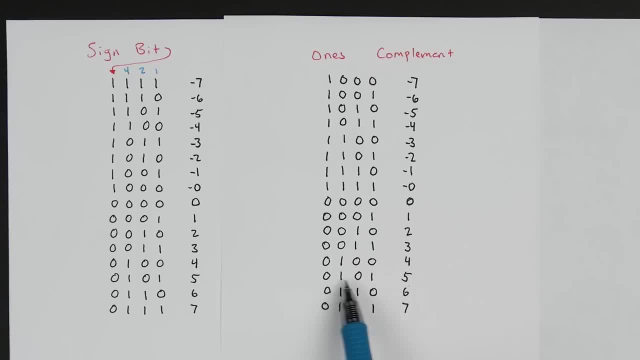 And so on. If you look at each of these numbers, So 5 is 0, 1, 0, 1.. Negative 5 is 1, 0, 1, 0.. So what happens with this? 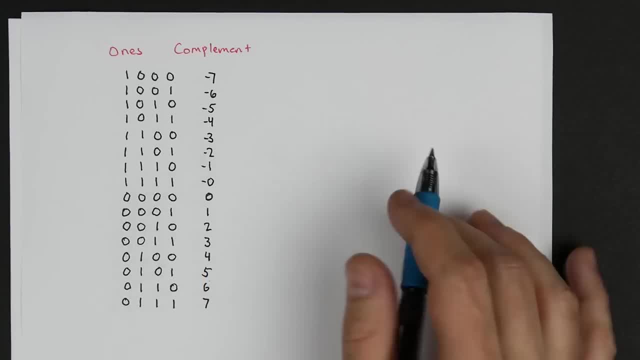 So we still have this kind of strange thing where we have negative 0. And we'll come back to that in a minute. But what we can do is we can try to, you know, add some numbers. So if we add 5.. 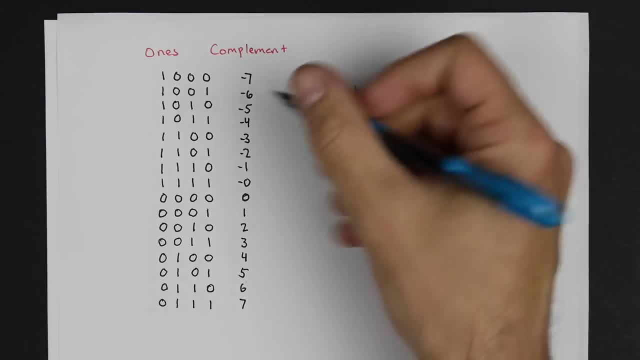 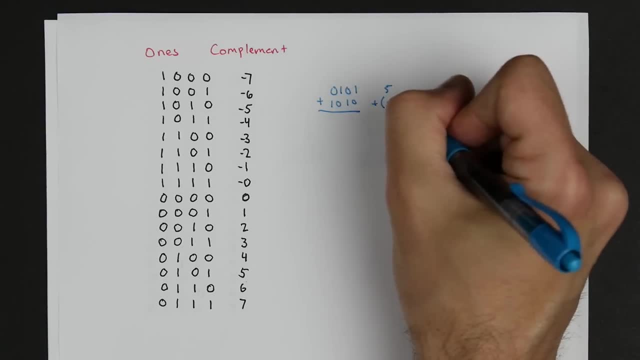 So 0, 1, 0, 1. So that's 5. And negative 5. 1, 0, 1, 0. So if we do those adding negative 5 here, what we end up getting is 1 plus 0 is 1.. 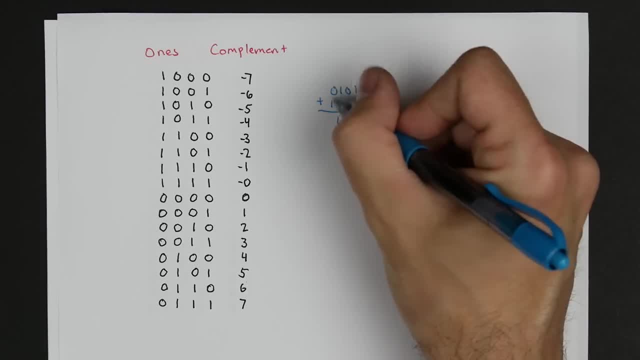 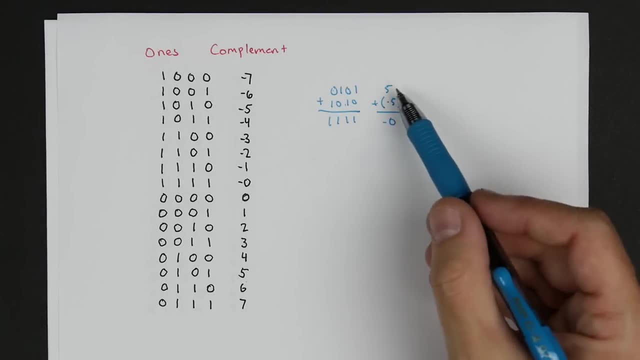 0 plus 1 is 1.. 1 plus 0 is 1.. 0 plus 1 is 1.. We get 1, 1, 1, 1, which is negative 0. So that's closer right. 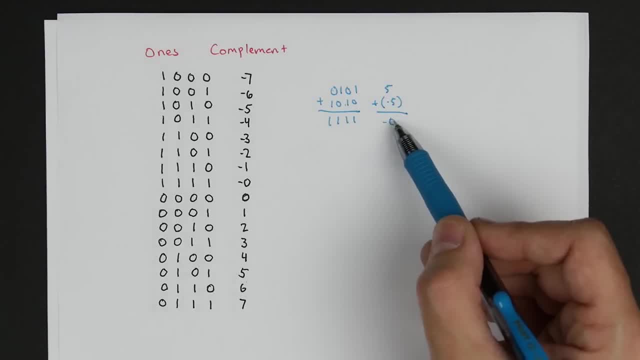 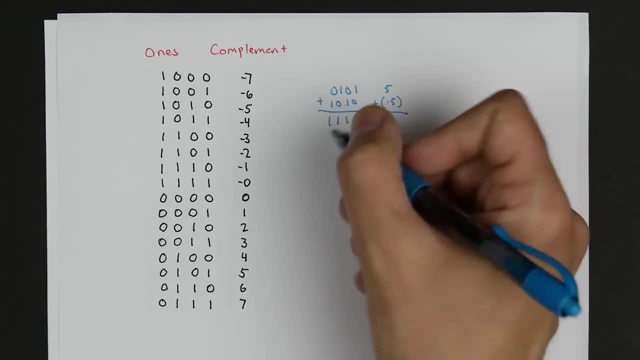 You know, 5 minus 5, you'd expect to get 0. Negative 0 is, I guess, the same thing. So that's pretty good And that actually works for any of these. You know we can do 3 minus 3.. 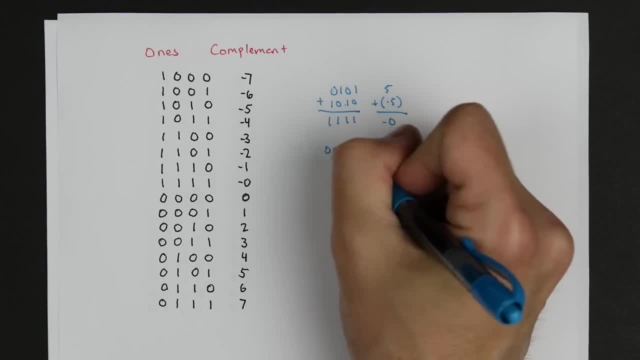 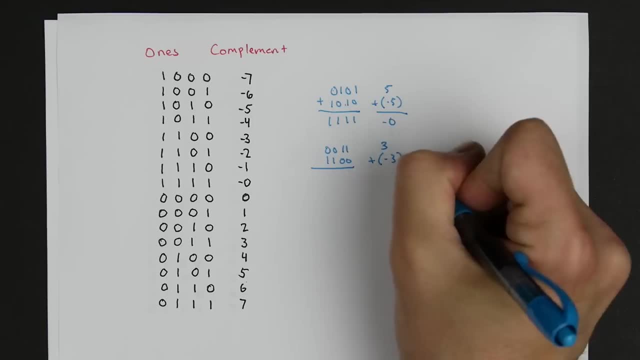 So 3 is 0, 0, 1, 1.. Negative 3 is 1, 1, 0, 0.. So this is 3 plus negative 3 if we add these together. So 1 plus 0 is 1.. 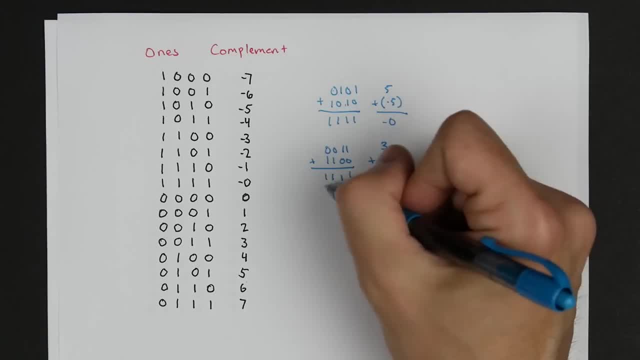 1 plus 0 is 1.. 0 plus 1 is 1.. 0 plus 1 is 1.. We get 1, 1, 1, 1 again, And so again: 3 minus 3 is negative 0.. 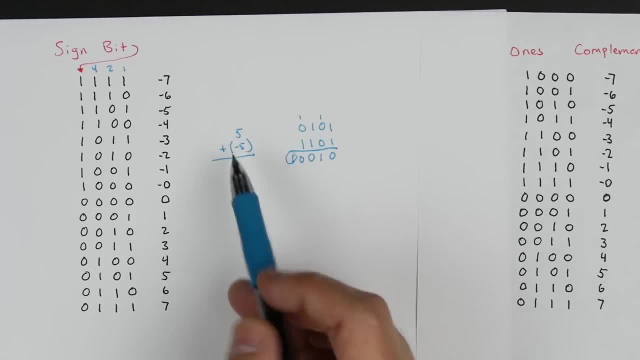 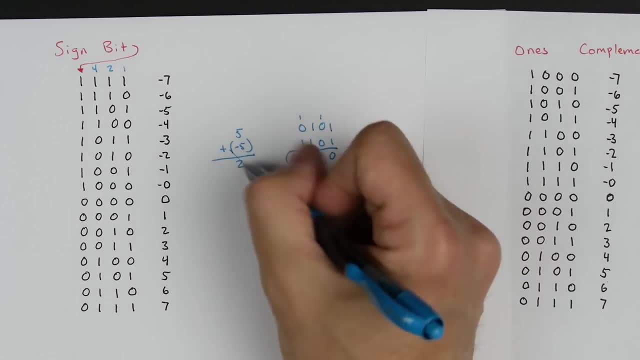 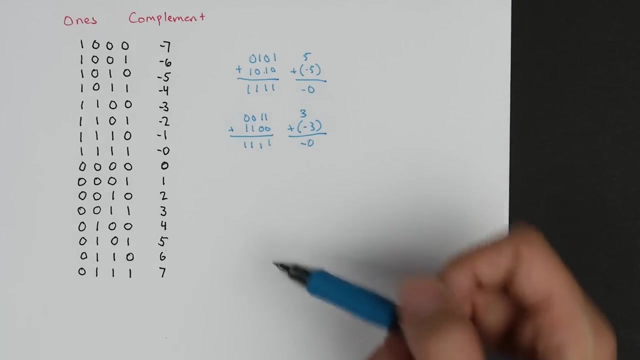 So this is definitely doing a lot better than here, where we were seeing 5 minus 5.. Minus 5 was 2.. That's definitely not right. So negative 0, definitely a lot closer. Let's try some other things, kind of see if we can see a pattern here. 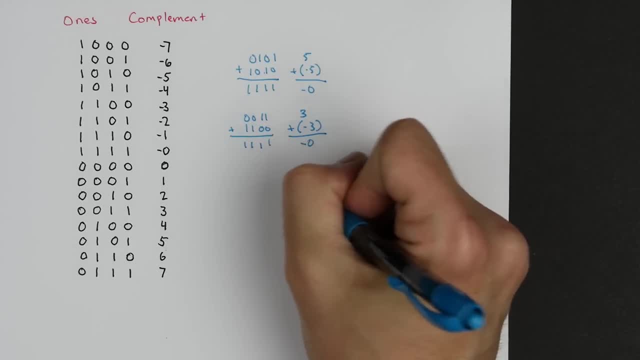 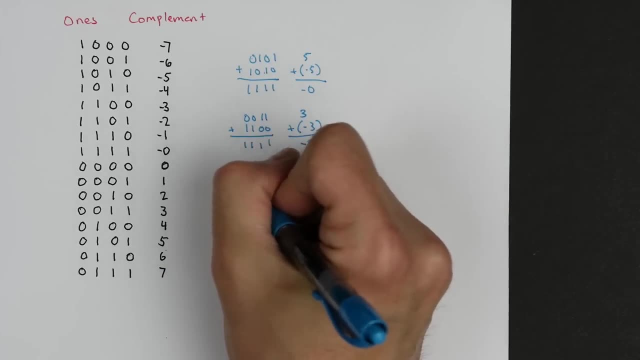 So if we did, let's say, 5 plus negative 3.. So 5 minus 3, let's see what we get there. So 5 is 0, 1, 0, 1.. And negative 3 is 1, 1, 0, 0.. 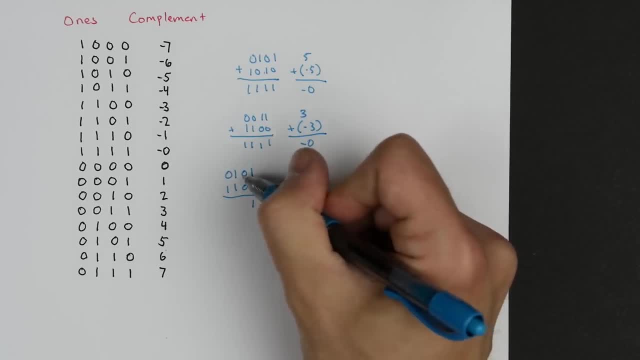 So 1 plus 0 is 1.. 0 plus 0 is 0.. 1 plus 1 is 2.. So we'll put a 0 and carry a 1. And then 1 plus 1 again is 2.. 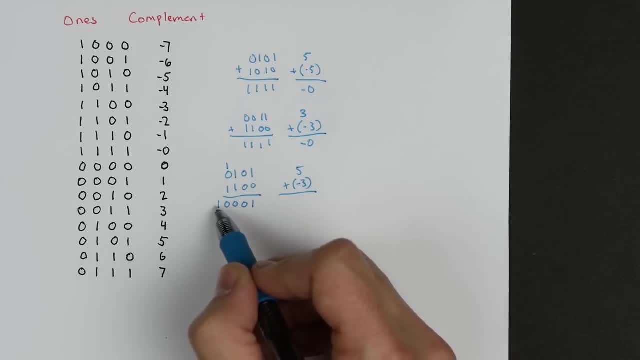 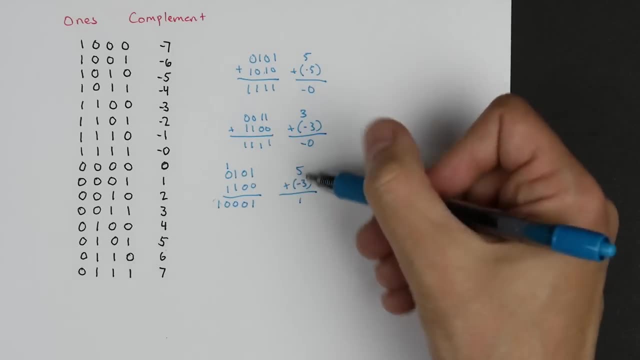 So we'll put a 0 and carry a 1.. And so if we ignore this first bit here, because we're working with 4 bits, we get 1.. So 5 minus 3 is 1.. That's close. 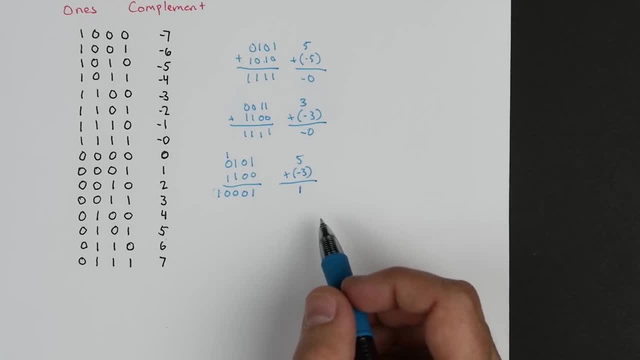 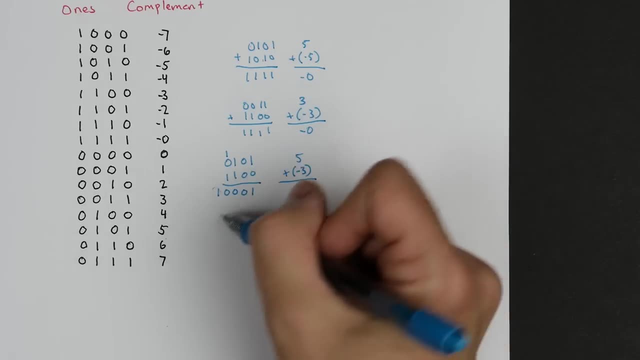 It should be 2, but you know, let's see what happens if we do. let's say 6 minus 2.. Or 6 plus negative 2.. So 6 is 0, 1, 1, 0.. 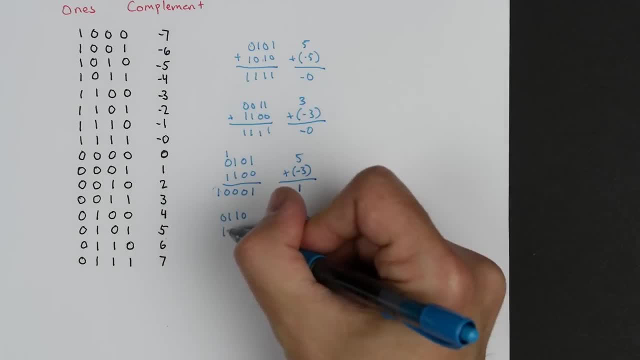 Negative: 2 is 1, 1, 0, 1.. 1, 1, 0, 1.. 0 plus 1 is 1.. 1 plus 0 is 1.. 1 plus 1 is 2.. 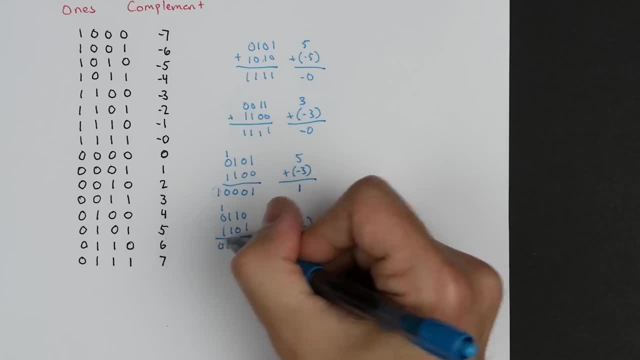 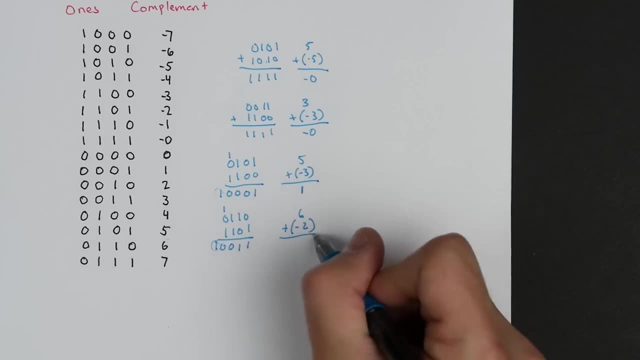 Put a 0 and carry the 1.. 1 plus 1 is 2.. Put a 0 and carry the 1.. Again, ignore that first bit, because we're working with 4 bits. So 0,, 0, 1, 1 is 3.. 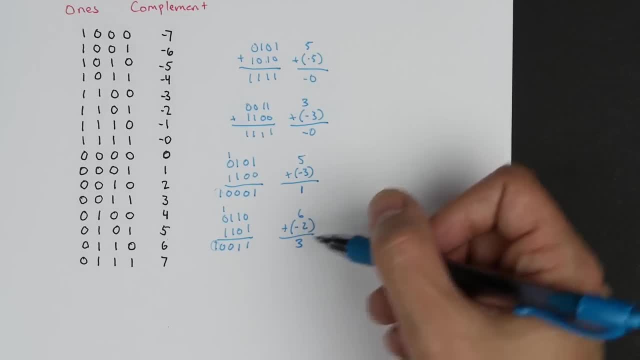 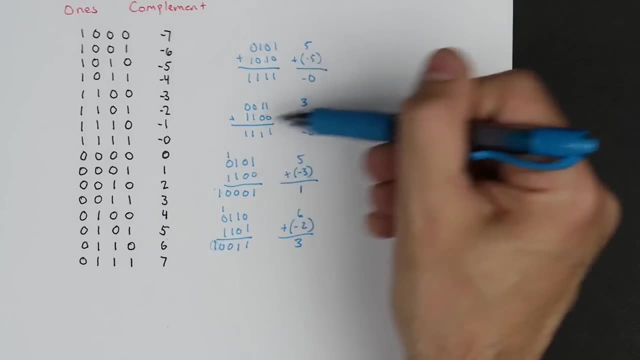 So we're saying 6 minus 2 is 3.. Close, But we're definitely seeing an interesting pattern here. In fact, if we look, you know these places where we're getting this negative 0, if we just go down 1, we see 0.. 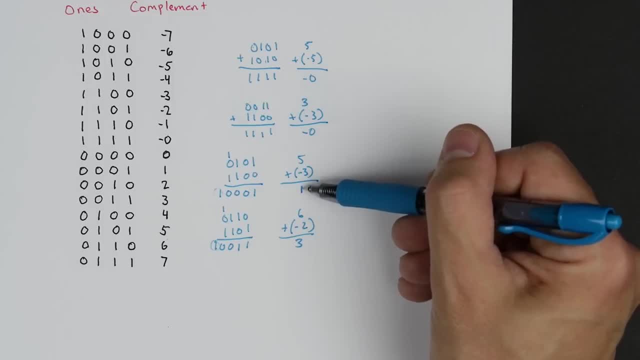 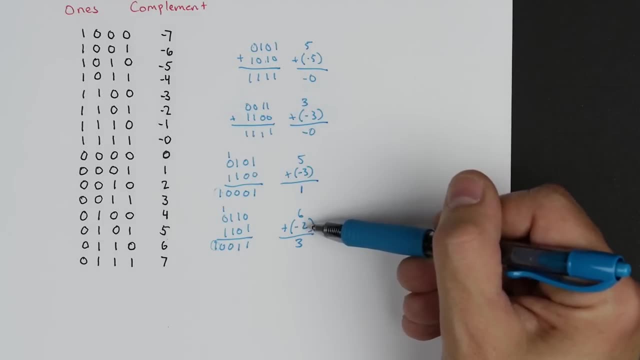 Which is what we want Here. 5 minus 3,: we'd expect to see 2,, but we're seeing 1.. So if we just go down 1, we'd actually see a 2.. 6 minus 2,: we'd expect to see 4,, but we're actually getting 3.. 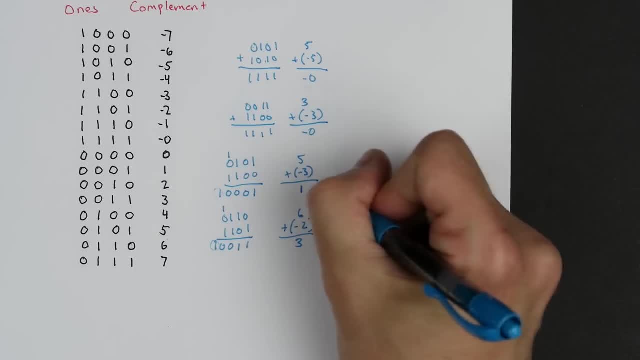 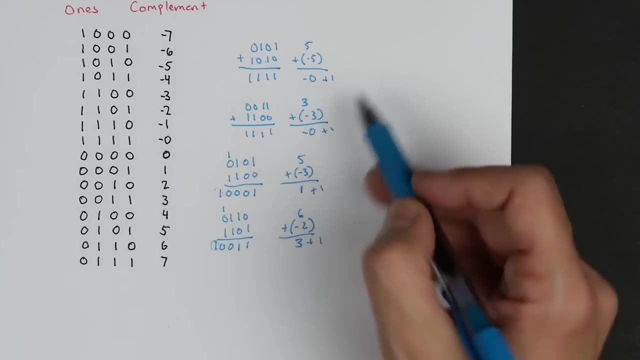 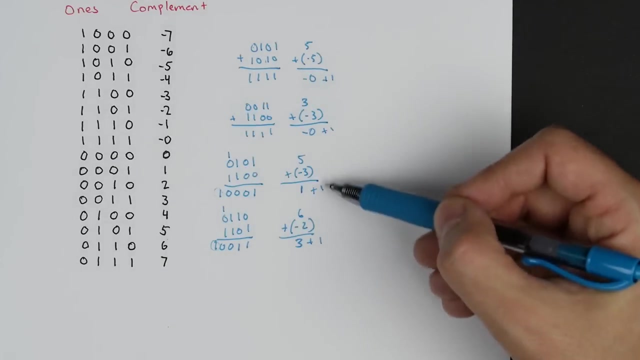 But if we go down 1, we get the right answer. So we could just always add 1 to each of these. Of course it's kind of weird to say add 1 to negative 0 to get to 0. But if you kind of bear with me a minute, you'll see that if we add 1 to the binary value and it flips over, you do get to the right thing. 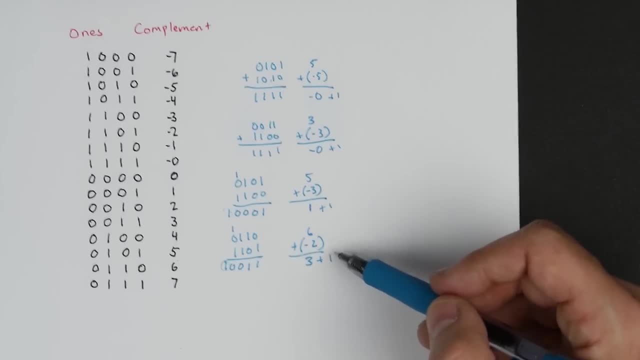 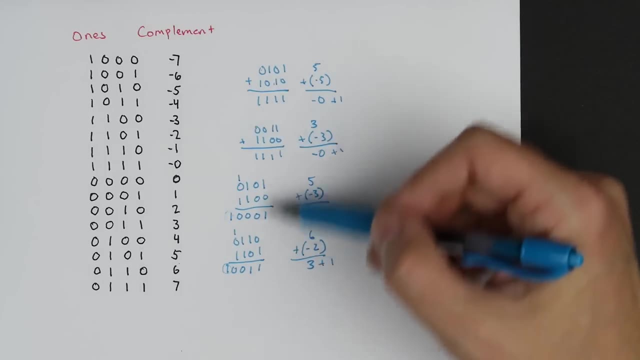 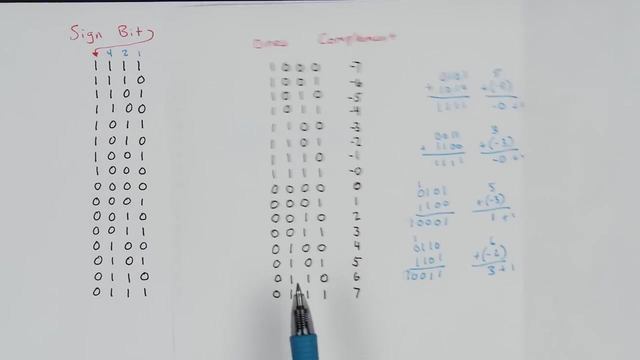 And here you get to the right thing. So the ones complement. you know, just flipping all of these bits is close, It's very close. It's off by 1 on all of our arithmetic And it also still has that nice property that we saw with the sign bit, which is, you know, you can look at this first bit and you can tell these are all negative numbers. 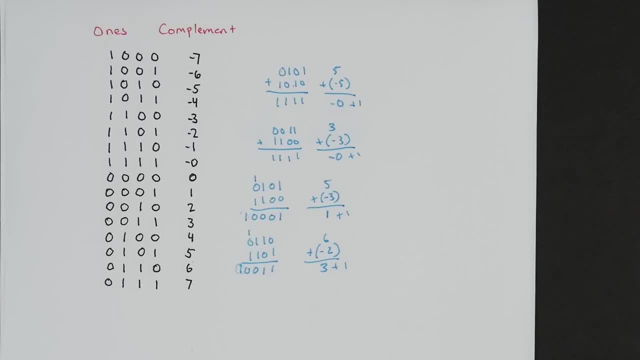 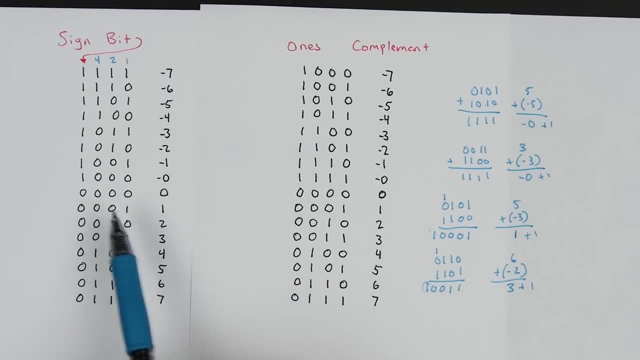 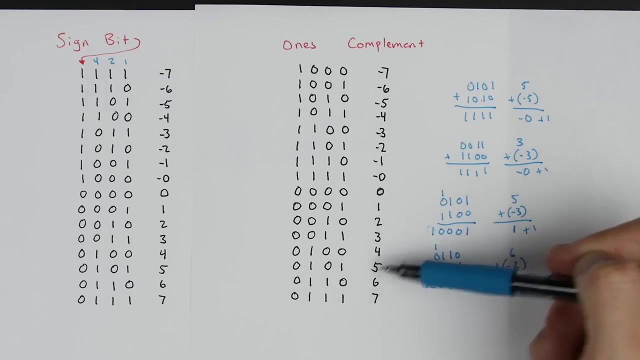 And if the first bit is 0, then they're positive numbers. So it seems like the ones complement has a lot of the you know a lot of nice properties. you know that you'd have in the sign bit. The one thing that's you know well, I guess it's not too bad- is that to get from to negate a number, you know if you're going from 5 to negative 5 with a sign bit. 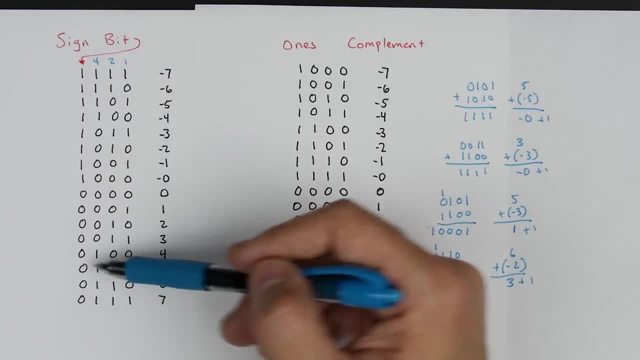 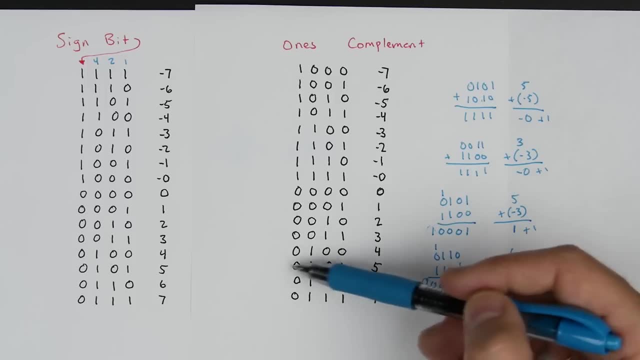 all you'd have to do is flip one bit. You just flip that first bit to a 1 and you get to negative 5.. With the ones complement you have to invert each bit, So it's a little bit more work. But of course inverting bits is pretty easy to do in hardware if we're building hardware to do this. 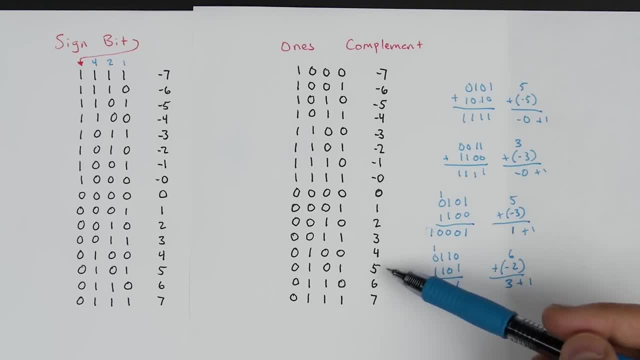 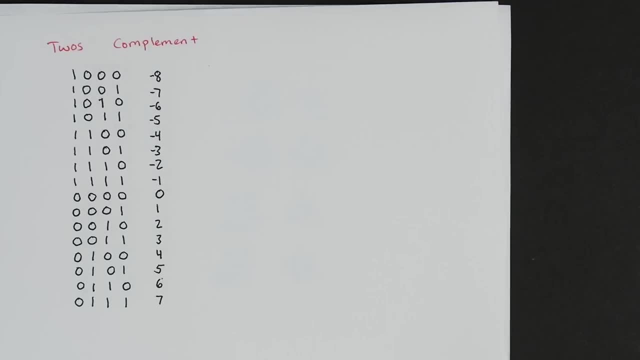 If we're building a computer it's going to be doing some math. So ones complement seems pretty good, but it is off by 1.. So what we can do is look at another scenario, which is twos complement, And if we compare ones complement to twos complement, 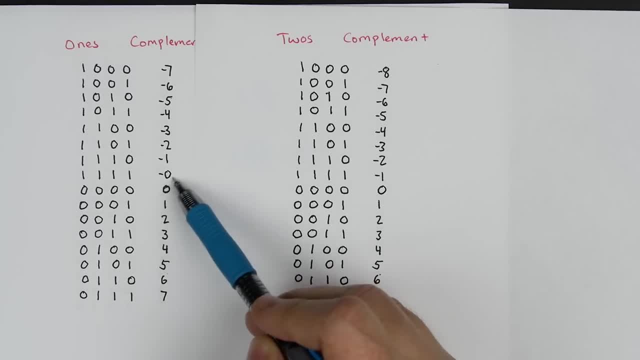 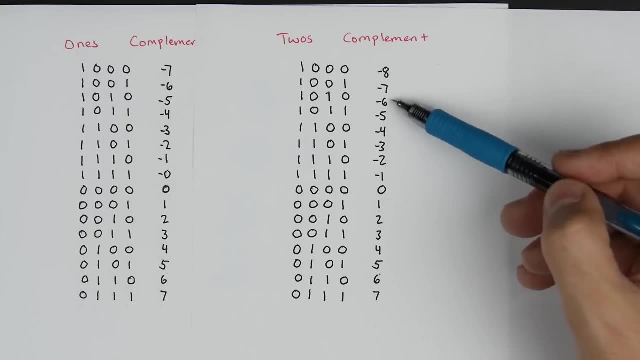 it's basically the same, except what it does is it gets rid of this negative 0. So instead of having negative 0, we just go right to negative 1.. Negative 2,, 3,, 4,, 5,, 6,, 7.. 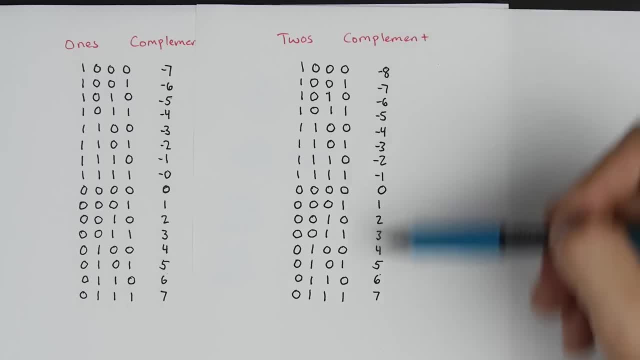 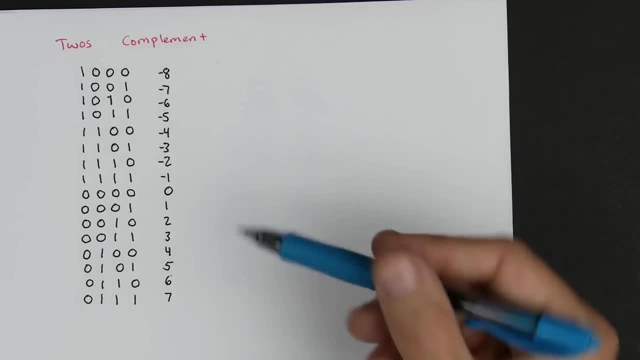 And the kind of weird thing here is we have a negative 8. And we don't have an 8. But the nice property about this is that all of our math works out very nicely. So if we have 5 minus 5,, 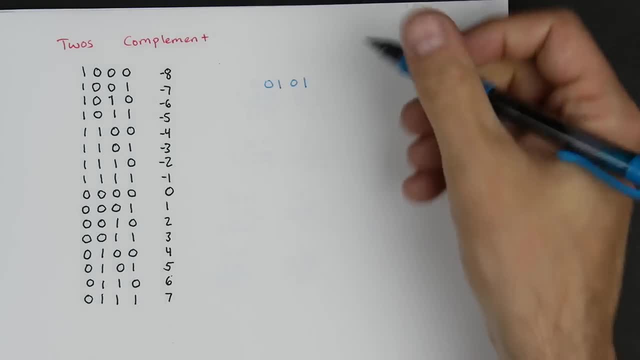 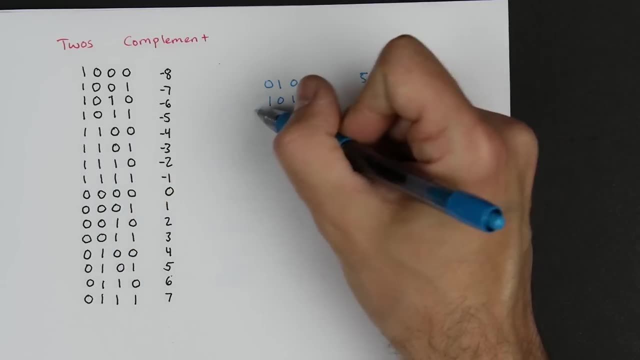 5 here is 0, 1,, 0, 1.. And so that's 5.. And negative 5 is 1, 0, 1, 1.. So 1, 0, 1, 1.. 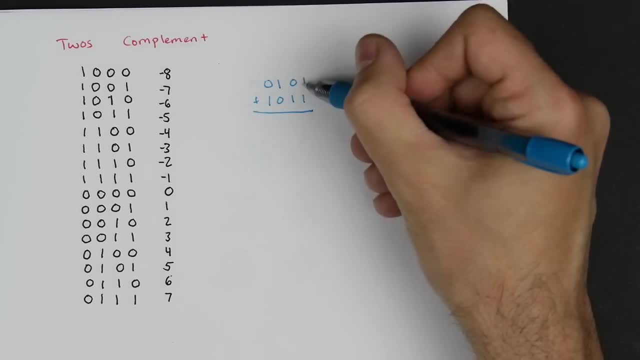 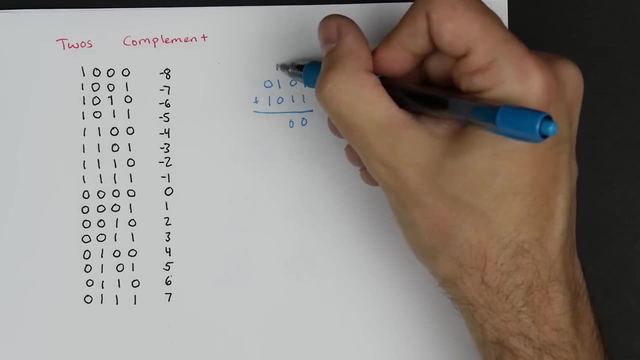 And if we add these things, if we add negative 5, 1 plus 1 is 2.. So we'll put a 0 and carry the 1.. 1 plus 1 is 2.. Put a 0 and carry the 1.. 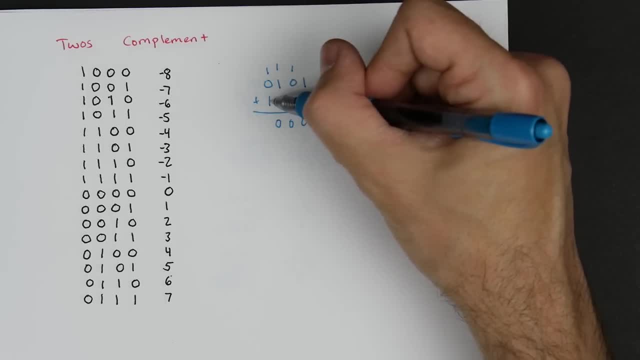 1 plus 1 is 2.. So we'll put a 0 and carry the 1., And 1 plus 1 is 2.. So put a 0 and we have a 1 that we're carrying, And so you'll notice that each. 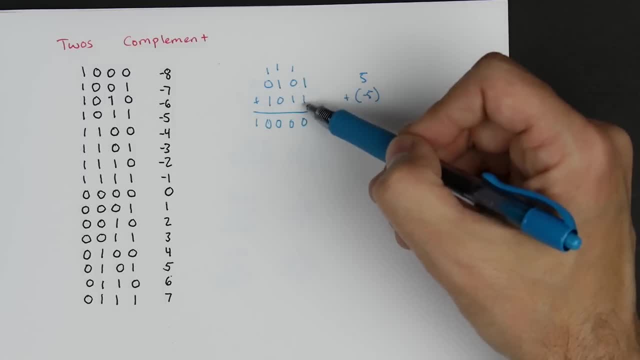 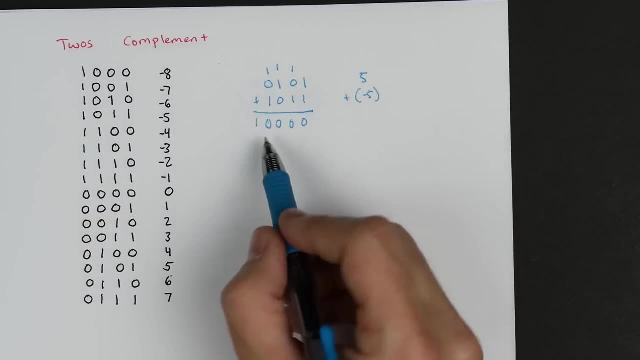 when we're looking at the negated version of something. when we add each of these place values, we get a 2 each time, And that's why it's called 2's complement. But in any event, you see that we end up with 0,. 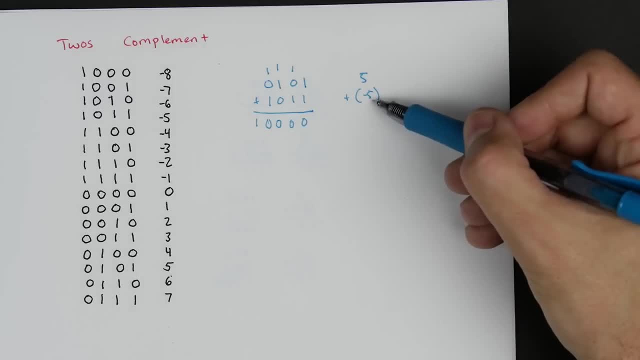 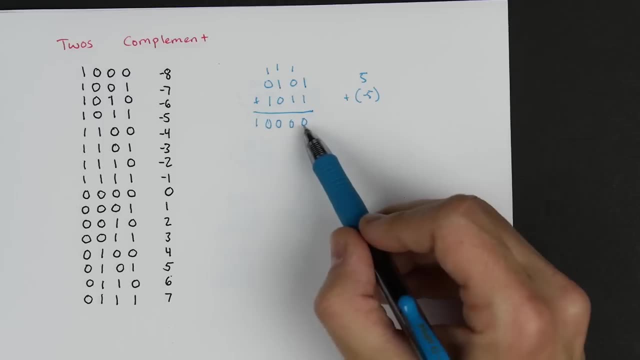 which is just what we would want- when we add a number to its inverse- And in fact you can try it with any of these numbers and you'll find out that you get all 0s. So let's try. you know, 6 minus 2.. 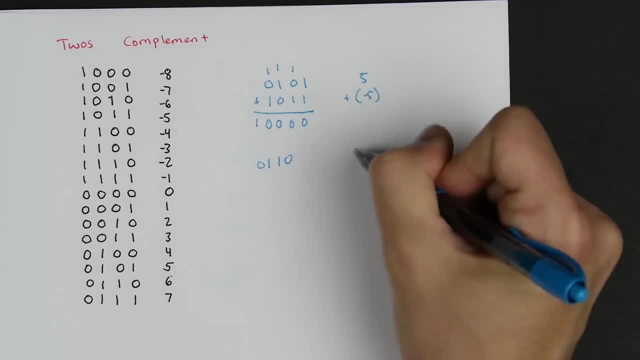 So 6 is 0, 1, 1, 0.. That's 6.. And a minus 2 is 1, 1, 1, 0.. 1, 1, 1, 0.. 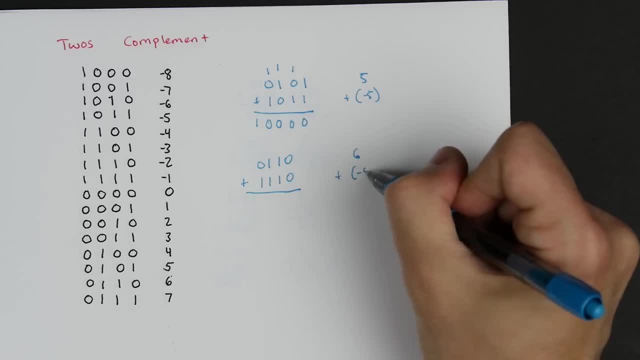 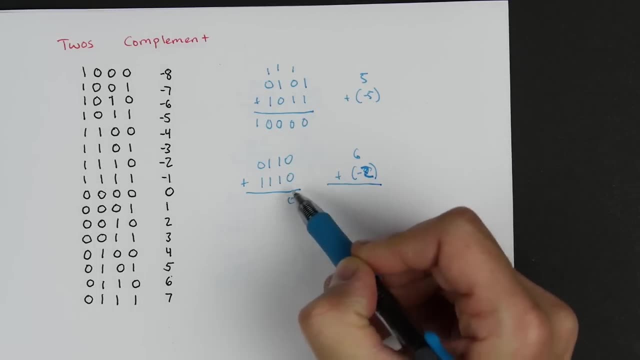 And if we add these together, so if we add our negative 2, whoops, negative 2.. Adding negative 2 there: 0 plus 0 is 0.. 1 plus 1 is 2.. So we'll put a 0 and carry the 1.. 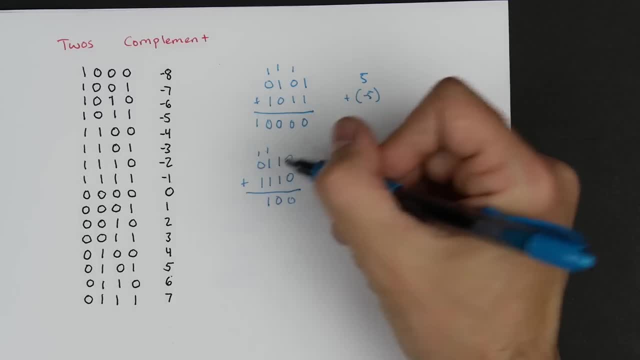 1 plus 1 plus 1 is 3.. So that's a 1 and a carry a 1.. And the 1 plus 1 is 2.. So 0 and carry a 1.. And again, we ignore that. 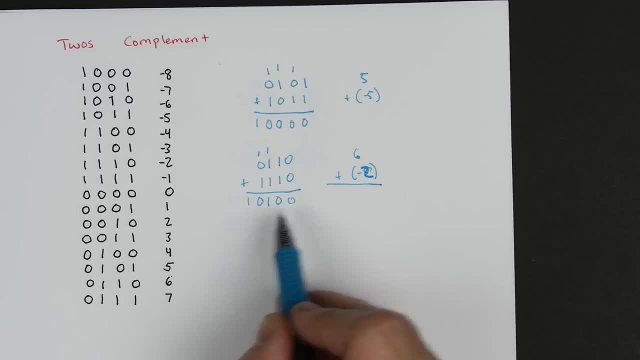 Fifth bit there, And so 0, 1,, 0, 0 is 4.. And sure enough, 6 minus 2 should be equal to 4.. So this 2's complement works pretty well, And it also has this nice property again. 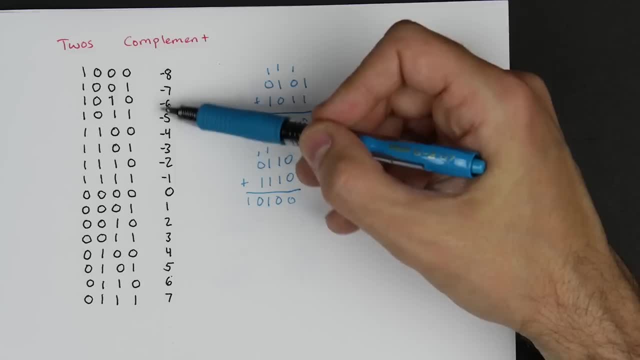 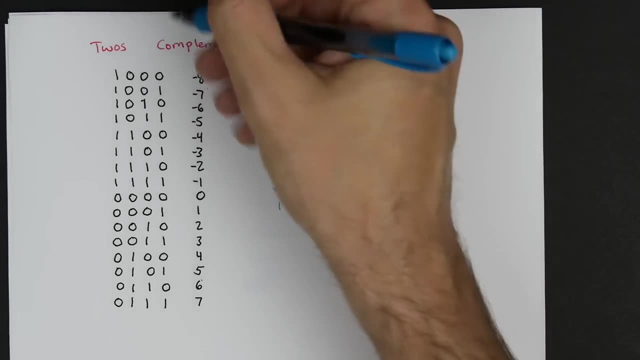 that that first bit is a sign bit right, Because all of these negative numbers have a 1 there. And what's even more interesting about 2's complement is, if you look at the place values, it actually makes sense. This is our 1's place. 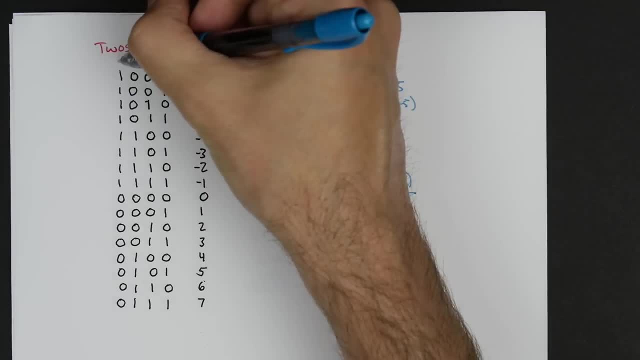 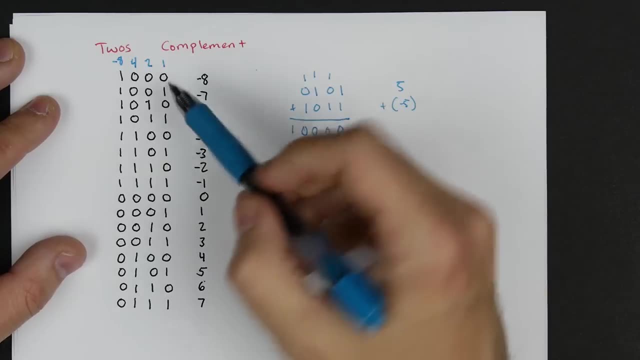 This is our 2's place, This is our 4's place And this place, here it's. you know it looks like a sign bit, but really it's a negative 8's place And you can see when we have a negative 8 in all 0's. 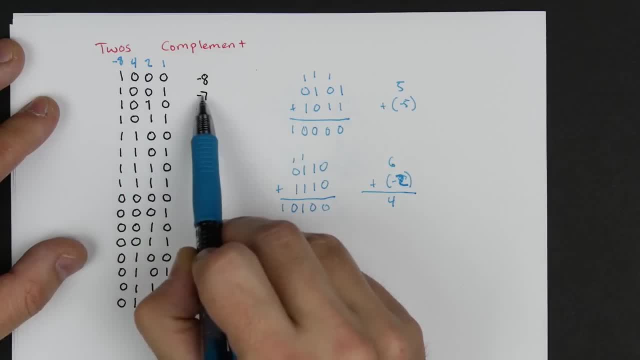 we have a negative 8.. But if you have a negative 8 and a 1,, you get negative 7, right. If you have negative 8 and a 4,, you get negative 4.. If you get negative 8 plus 4 plus 2 plus 1,. 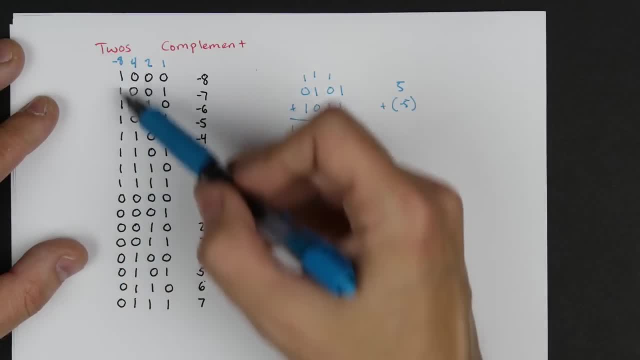 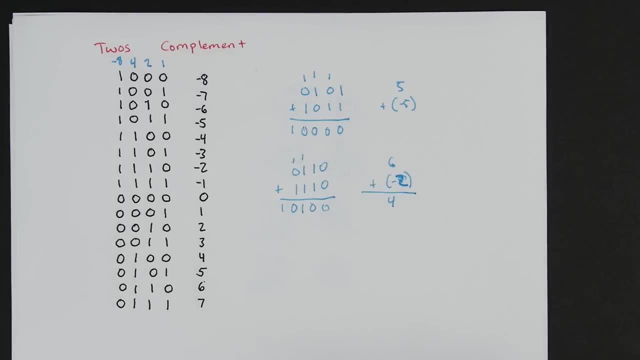 you end up at negative 1.. So this bit value actually has a mathematical meaning, which is why our math works out. So it's pretty cool. The one thing that's a little bit harder with 2's complement is negating a number. 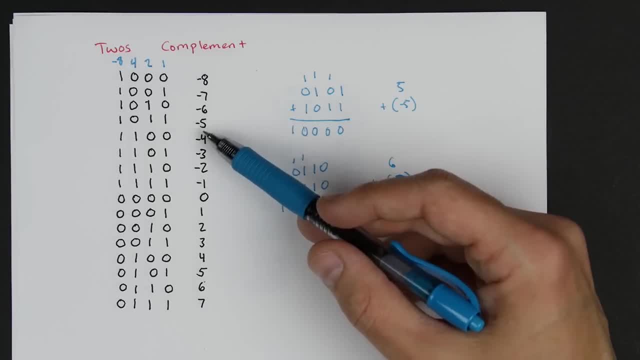 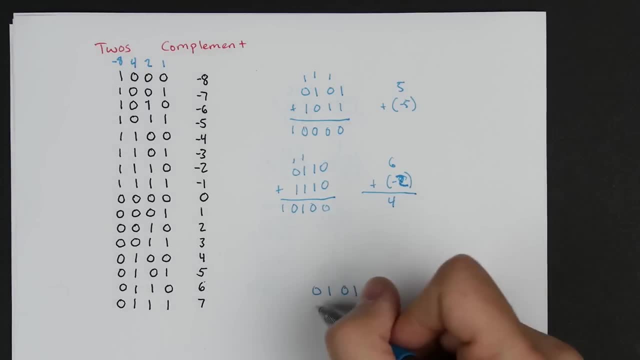 So if we want to go from a 5 to a negative 5, it's kind of a two-step process, right? So 5 is 0, 1,, 0, 1.. The first thing you have to do is take the 1's complement. 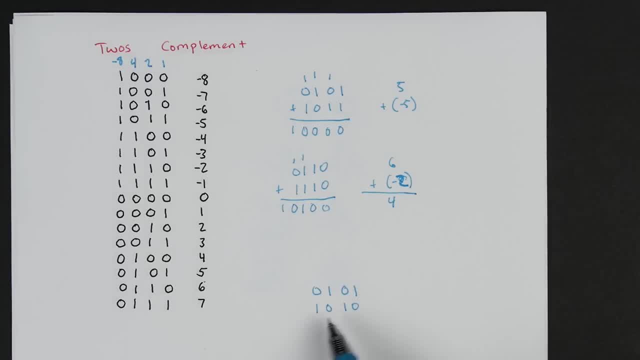 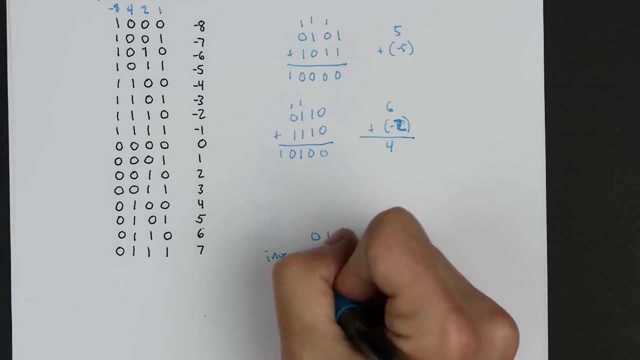 1, 0, 1, 0.. So flip all the bits So you're just inverting everything. That's easy enough. But then you have to add 1.. So you invert And then add 1.. So to add 1 to 0, 1, 0, 1,.